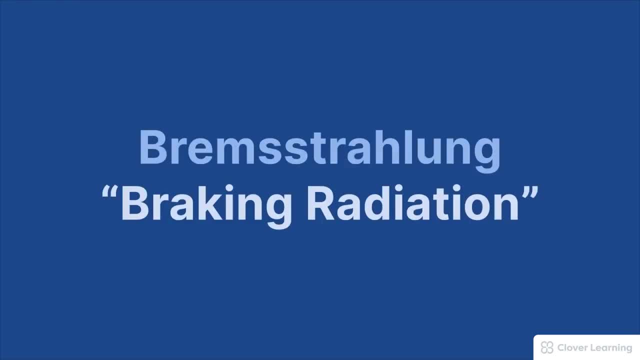 has a name. It's actually called bremstrelung radiation. This process has a name: It's actually called bremstrelung radiation. This process has a name: It's actually called bremstrelung radiation. This process has a name: It's actually called bremstrelung radiation. Bremstrelung. 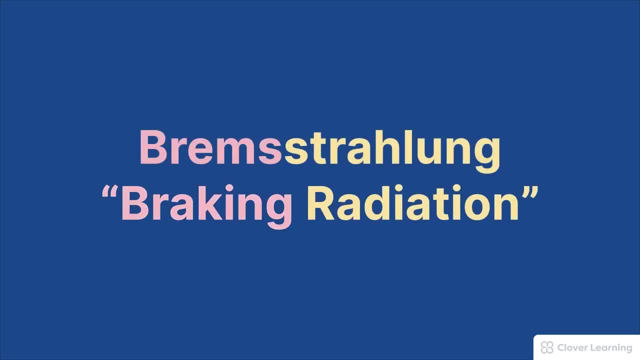 is the German word. that means breaking radiation, And that makes sense because the radiation is created because the electrons break or slow down. So you can kind of think of it like this: If you throw a ball at a glass window, the ball will slow down, and usually 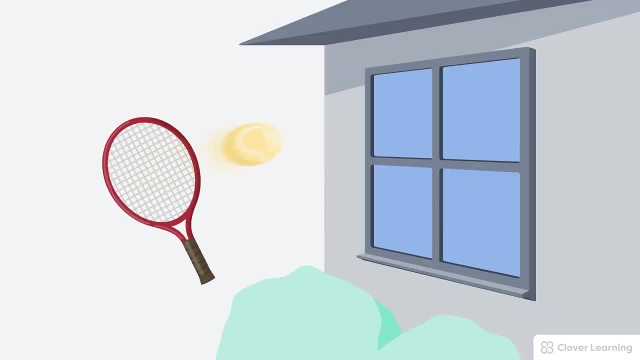 get deflected into another direction, just like when the electrons pass through the tungsten nucleus. But what happened to all of the energy that the ball was carrying? It had to go somewhere. The law of conservation of energy says that energy cannot be created or destroyed. It can. 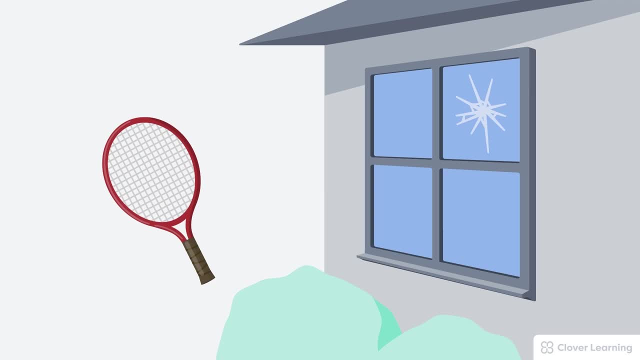 only change in form. So some of that original energy is left in the ball, but some of it leaves the ball and creates cracks in the glass. And this is just like how some of the electron energy leaves the electron and creates an x-ray photon- The energy of a bremsstrahlung radiation photon. 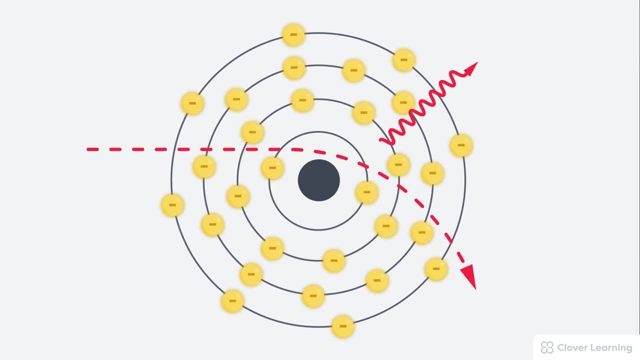 depends on a few factors, one of them being the energy of the incoming electron. If the incoming electron has an energy of 100 keV, the maximum energy photon that can be created is 100 keV. They won't always have the maximum energy, but they can. Here's another example: If the incoming 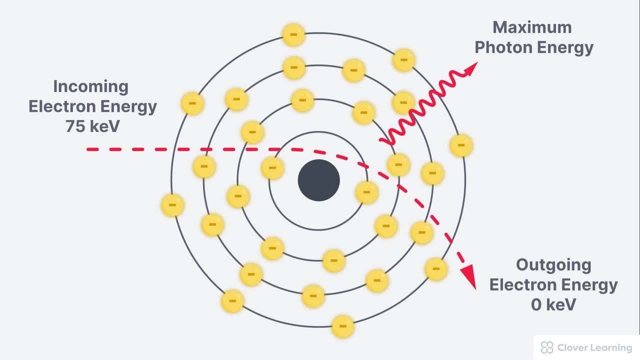 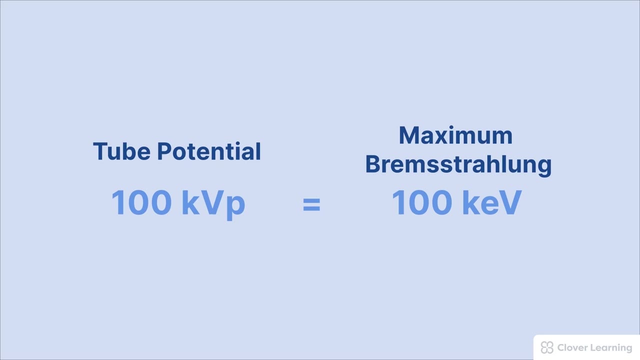 electron has an energy of 75 keV. the absolute highest energy photon that we can get out of that electron would be 75 keV. The maximum energy of a bremsstrahlung x-ray photon is controlled by the kVp, So the tube. 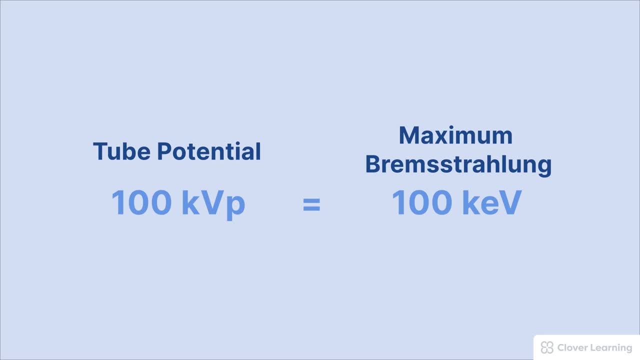 potential, if it's set to 100 kVp, will create bremsstrahlung photons that have a maximum energy of 100 keV And, of course, if we change the kVp, this changes If the tube potential is set to a. 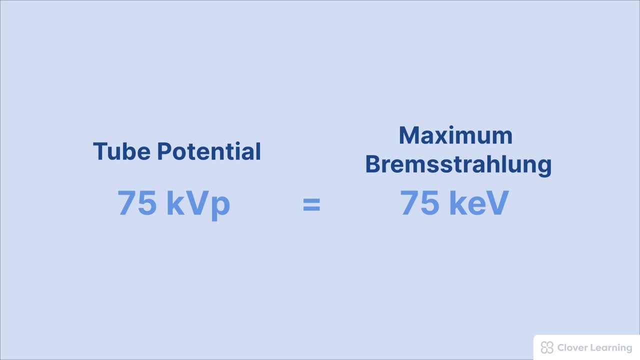 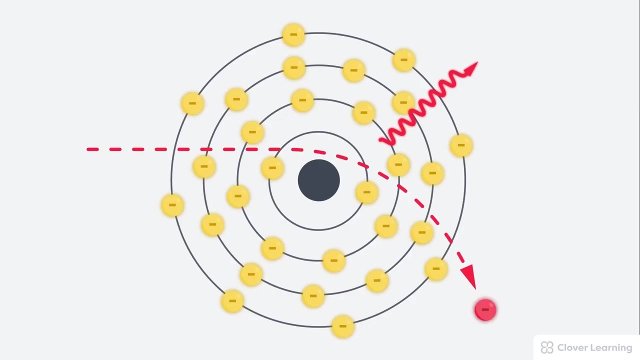 kVp of 75, the maximum bremsstrahlung x-ray photons will have an energy of 75 keV. Not many bremsstrahlung photons are going to have this maximum energy, And why is that? The energy of bremsstrahlung radiation also depends on how close the electron passes to. 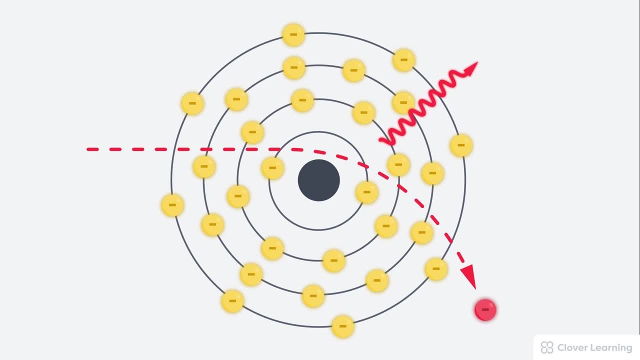 the nucleus. If the electron passes very close, as in this example, it will slow down significantly, change directions completely and give up most of its energy as an x-ray photon, For example, if the electron approaches with an energy of 90 keV, it will slow down to almost. 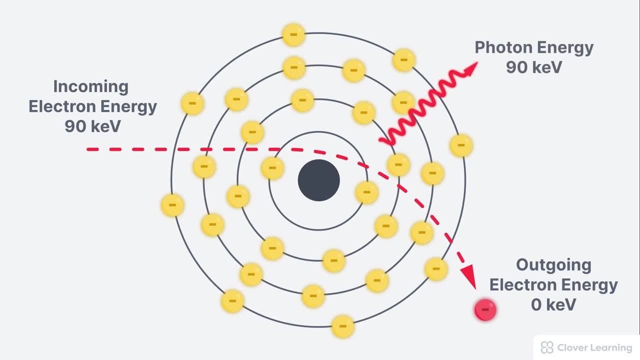 zero and release a photon with an energy of about 90 keV. But these electrons don't always pass very close to the nucleus. Here's another example. Let's say in this scenario the electron passes at a much greater distance from the nucleus and things will change. The attraction between the 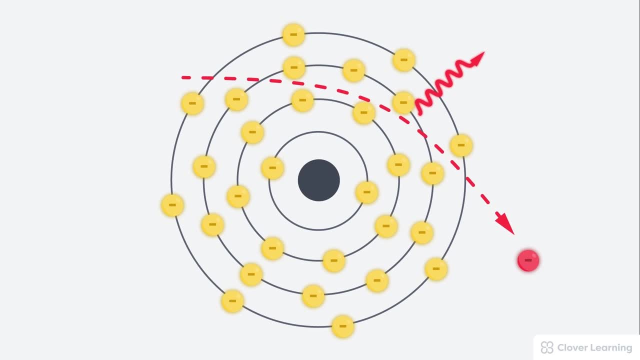 electron and the nucleus is weaker. The electron slows down some, but not completely. It changes direction some, but not completely, And it only gives up some of its original energy. For example, if the electron approached the x-ray photon, it would slow down some, but not completely. 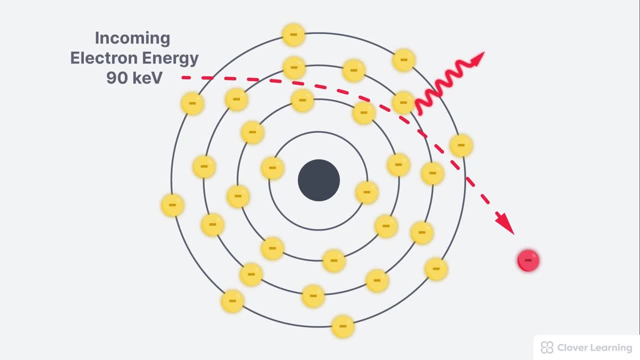 If the electron approached a certain atom with an energy of 90 keV but slowed down to an energy of 60 keV, the resulting photon would have an energy of 90-keV minus 60keV, which is 30 keV. All of the energy here is accounted for. 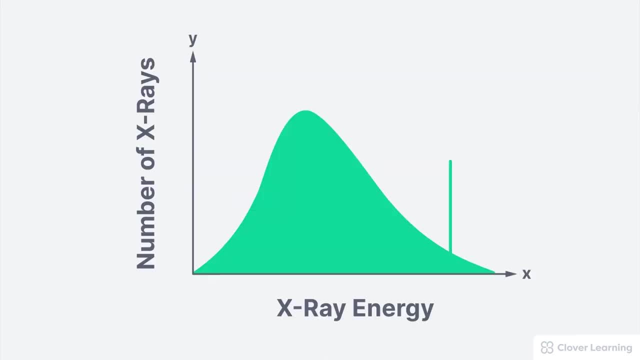 It is helpful to look at a graph of x-rays created during a single exposure. The x-axis is the different photon energies in the x-ray beam. The y-axis is the number of vectors in rotation photons with that energy. so the tallest part of the curve represents the photon energies that 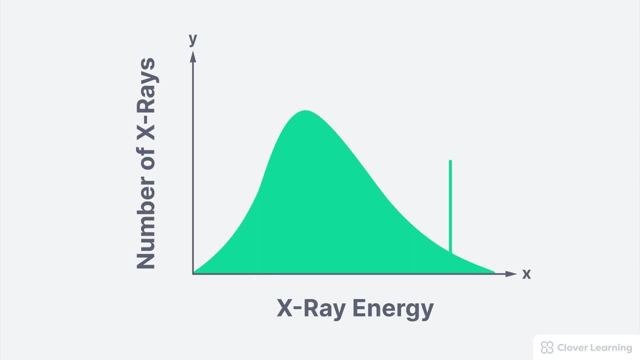 appear most often in the beam, The large bell curve, are the bremsstrahlung x-rays. A single exposure creates hundreds of millions of x-ray photons and almost all of these photons are bremsstrahlung x-rays. The curve is short on the left because most of the low energy bremsstrahlung 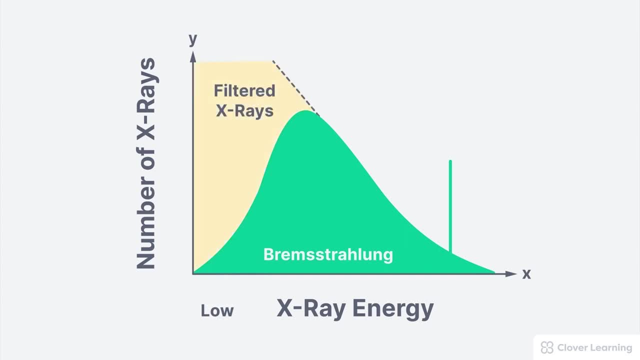 x-rays have been filtered out of the beam. These low energy photons came from electrons that slowed down not much at all. They can't penetrate the tissues of the patient, which is why they need to be filtered out. The curve is also short on the right because very few bremsstrahlung. 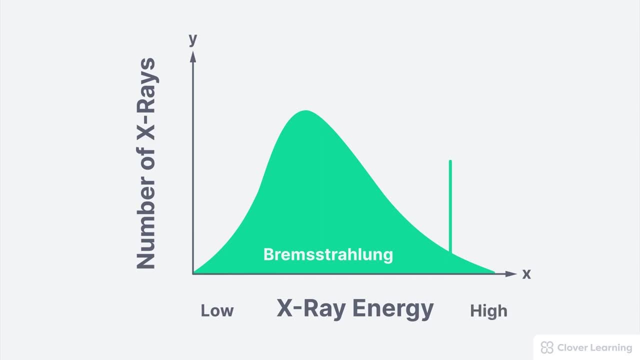 x-rays are created with the high energy. This comes from electrons that slow down to near zero and release all of their energy as a photon. The curve is tallest in the center because most of the delta x-rays are fired upstream. This is the color curve cause most of the resultant.